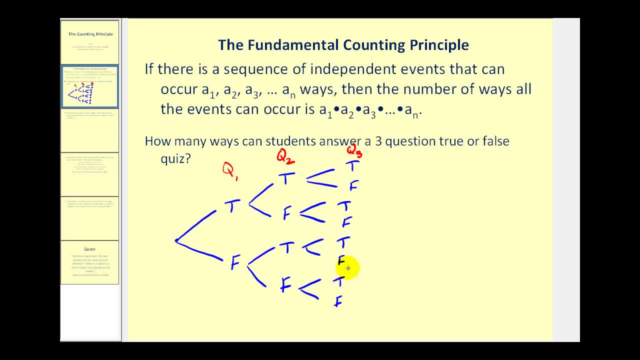 one, two and three for this quiz And you can see there are eight different ways: True, true, true, true, true, false, true, false, true, true, false, false, and so on all the way down this tree. Now it's much faster just to use the counting principle. 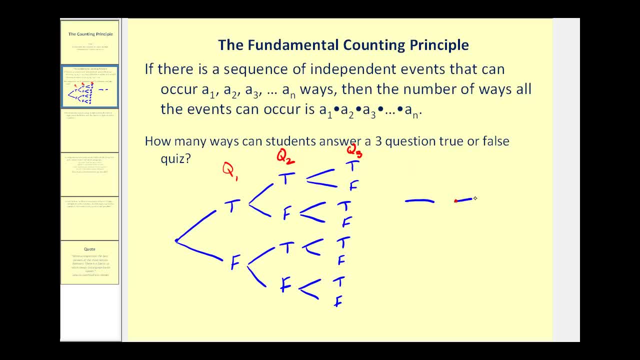 There are three events taking place here, one for each question, And each of these questions can be answered two different ways. So, using the counting principle, we'd have two times two times two for the first three questions, which equals eight possible ways this quiz can be answered. 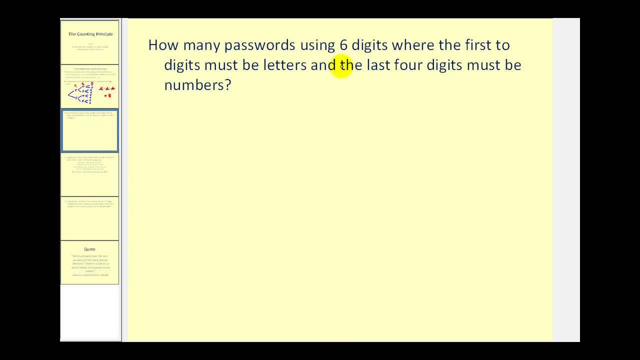 Let's take a look at another question: How many passwords using six digits, where the first two digits must be letters and the last four digits must be numbers? So there are six independent events here: One, two, three, four, five, six. The first two must be letters. 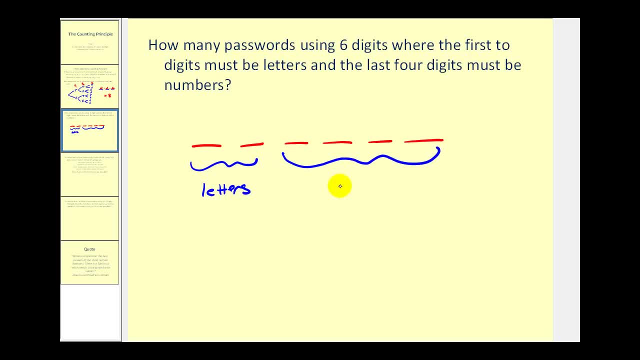 and the last four must be numbers. Well, there are twenty-six letters in the alphabet, so there's twenty-six ways. the first letter can be chosen, And the same for the second letter, And then the last four must be numbers. Well, the digits from zero to nine represent ten choices for each number. 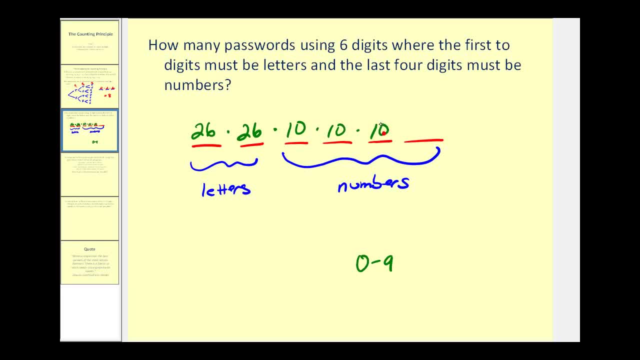 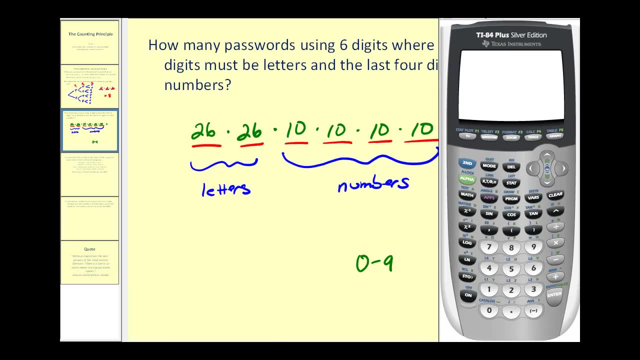 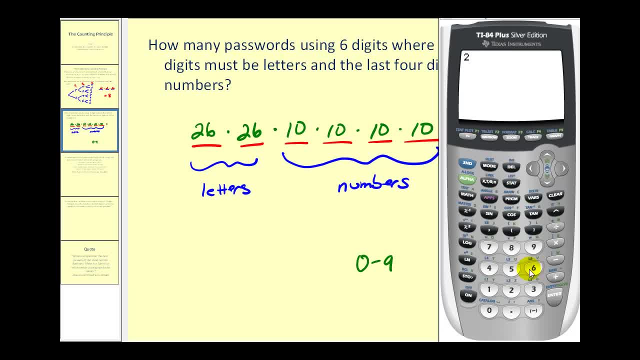 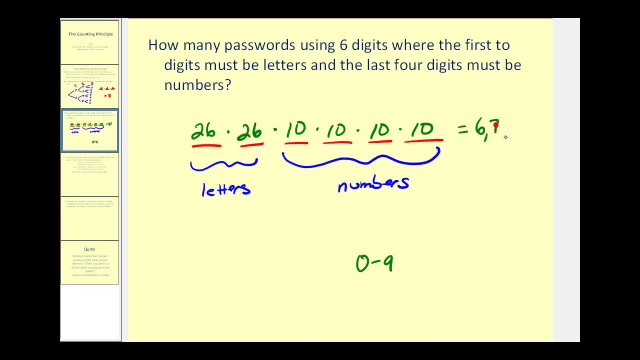 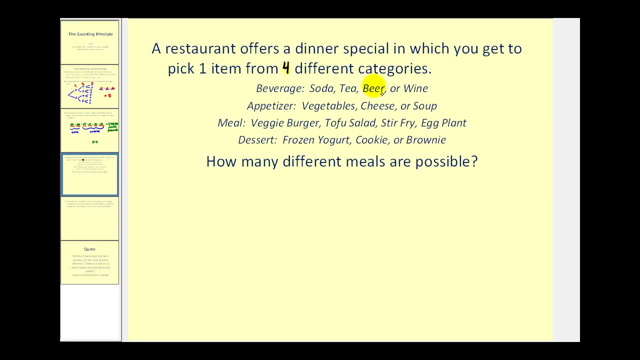 twenty-six squared times ten to the fourth, which equals six million seven hundred sixty thousand possible passwords. Let's go ahead and take a look at a couple more questions. A restaurant offers a dinner special in which you get to pick one item from four different categories, as we see listed here. 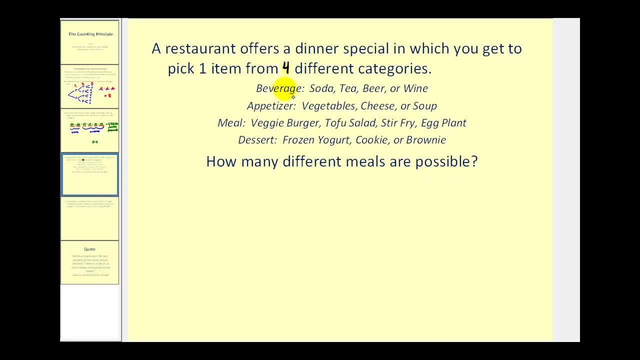 How many different meals are possible. First thing we should notice is we have four different categories to select from. So we have one, two, three, four independent events. So the first event would be for the beverage, second event would be for the 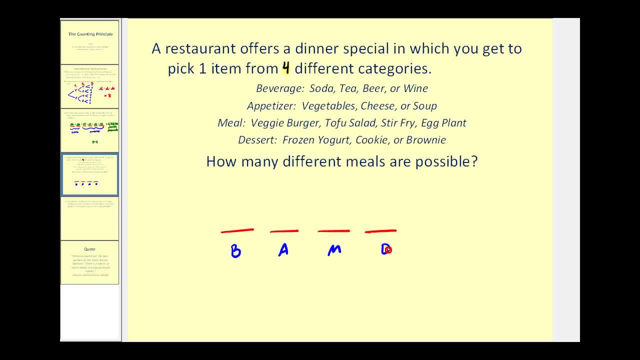 appetizer, third for the meal and fourth for the dessert. Looking at the beverage options, you can see there are four possibilities. So there are four ways that event can occur. For appetizers there are three. For the meal, there are one, two, three, four options. 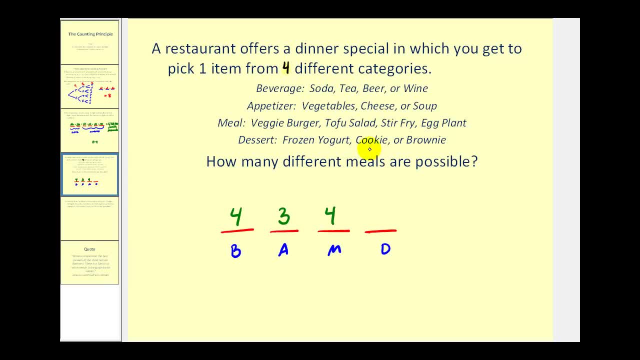 Or for ways to choose the main meal And for the dessert. we have three options, So the product of these will tell us the total number of ways we can select different dinners from this special. Four times three would be 12 times four would be 48 times three would equal 144.. So there are 144 ways. 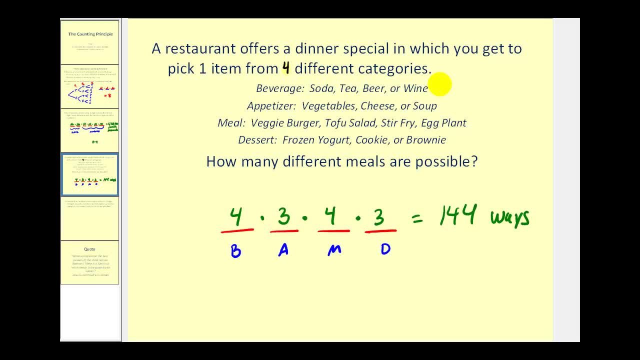 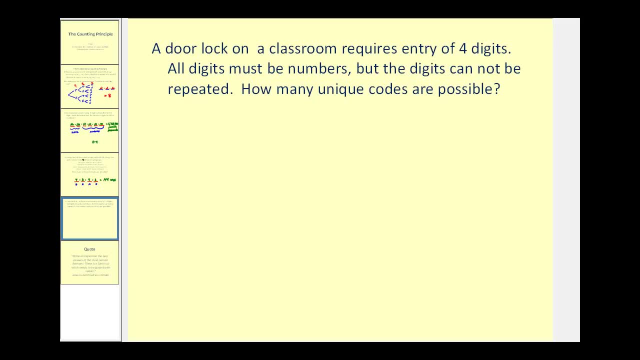 to select a dinner under these conditions. Let's go ahead and take a look at one more. A door lock on a classroom requires entry of four digits. All digits must be numbers, but the digits cannot be repeated. How many unique codes are possible? 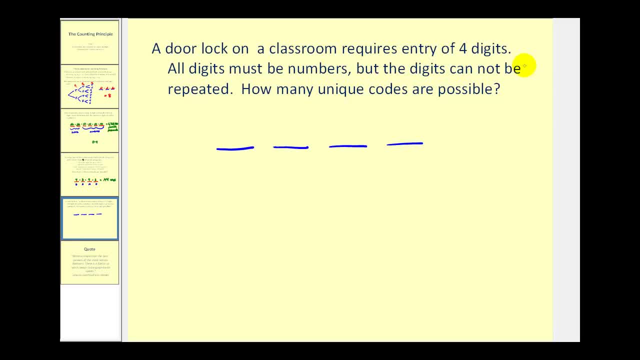 So again, this is very similar, except we do have a special condition here: that the digits cannot repeat. So it's a slight variation of the counting principle, since each of these digits are not independent because they cannot be repeated. However, for the first digit, 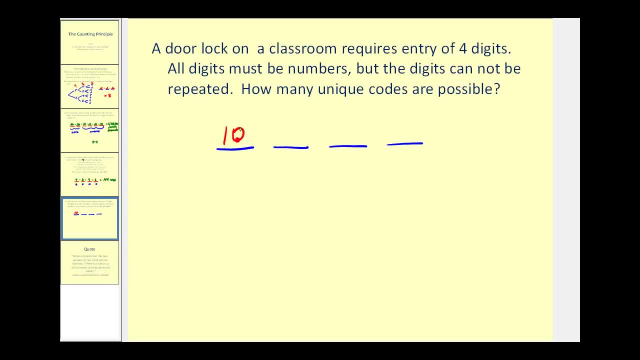 there are no restrictions. so there are 10 possibilities, zero through nine. But for the second digit we cannot repeat the digit used in the first position, So instead of 10 possibilities there would only be nine. And then for the third. 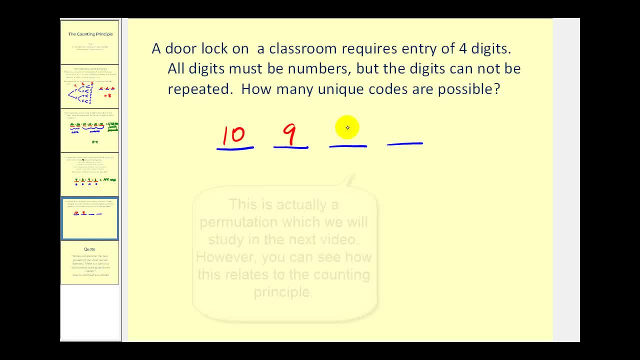 we can't repeat either of the first two digits, so that would leave eight possibilities. And then for the fourth, we can't repeat any of the first three, so that would leave seven possible digits. So the product of these would be the total number of unique codes that are possible. 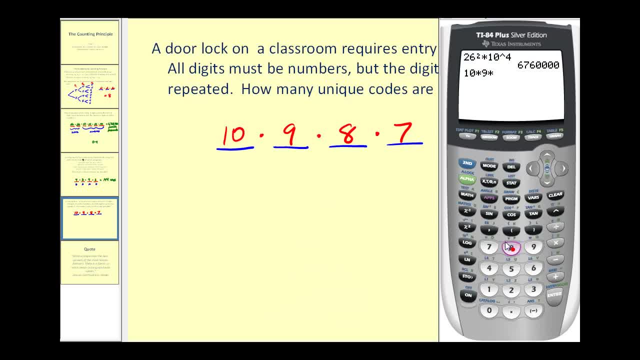 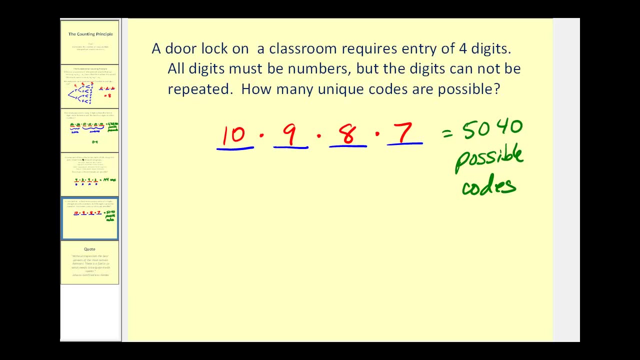 So we have 10, times nine times eight times seven, So there are 5,040 unique codes for the door lock. Okay, that'll do it for this video. Next we'll take a look at permutations and combinations. 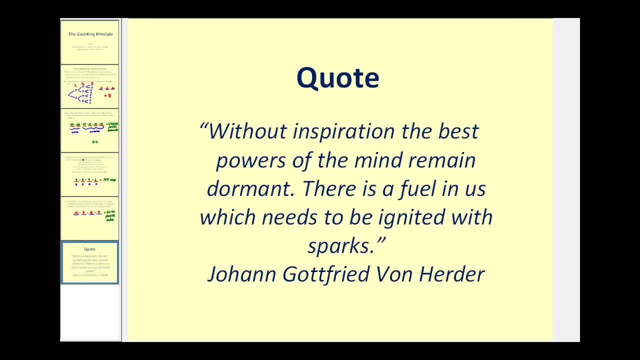 Thank you for watching. We'll see you in the next video.